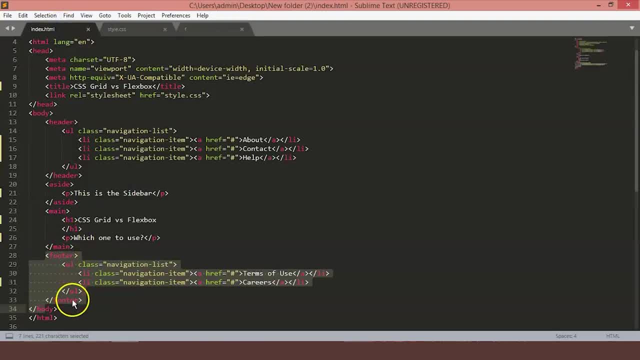 other. In the code you can see that this is the footer part of the page. this is the main content of the page, this is for the sidebar and this is for the header area of the page. For the styling part, we have used some basic. 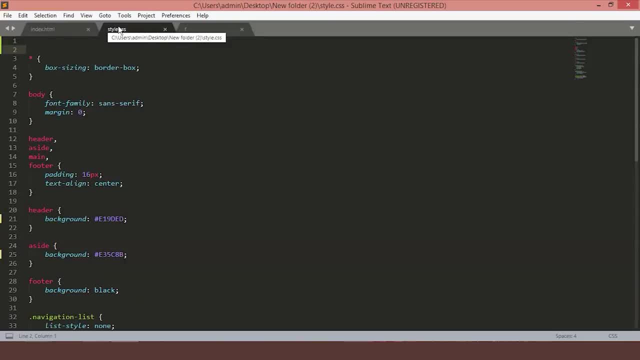 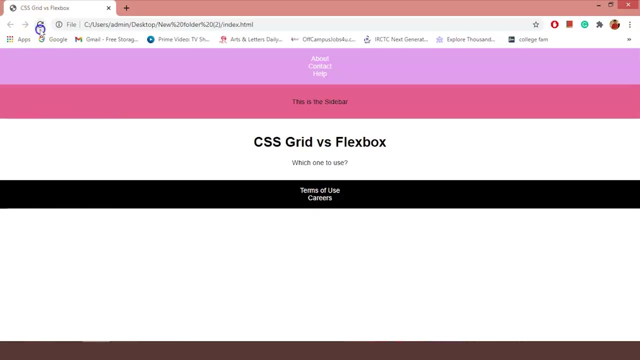 styling. just so as to understand the example better. Now we can turn the body into a grid by setting the display property to the grid. So here under the body, we will set the display to grid. Just save the file and refresh. You can see nothing changes because by default. 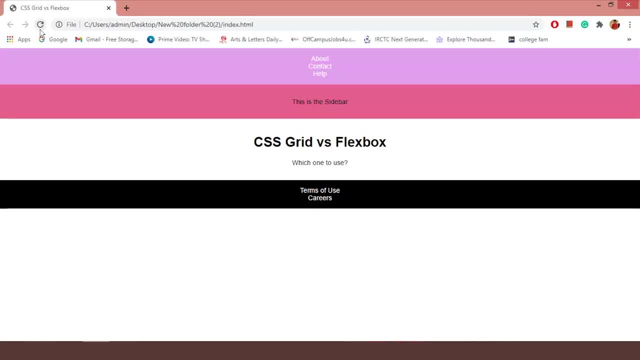 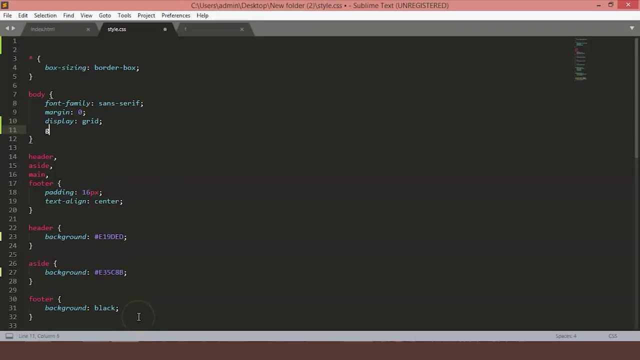 the CSS grid starts creating rows automatically and adds the content in these rows. That's why it didn't change. We can change it by adding the grid template column property in our body. In our case, we will need two columns: one for Sidebar and other for the Main Content. 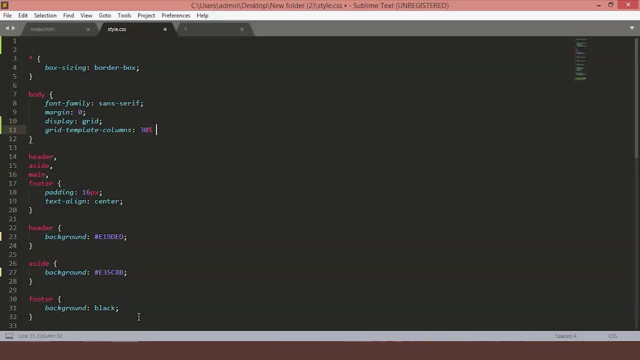 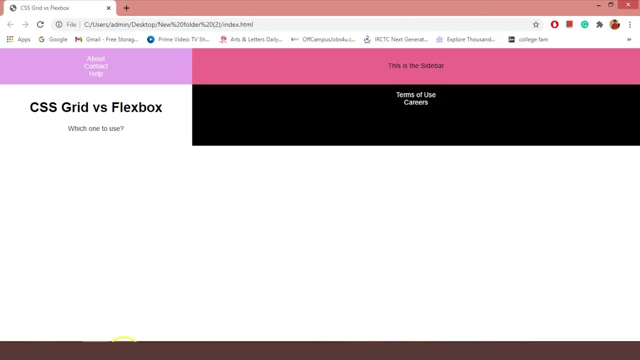 Let's set the side area to 30% and we will keep the main area to auto to cover the remaining spaces. Now if you save the file and reload, you can see the elements are broken into the cells we created. We will also define the content. 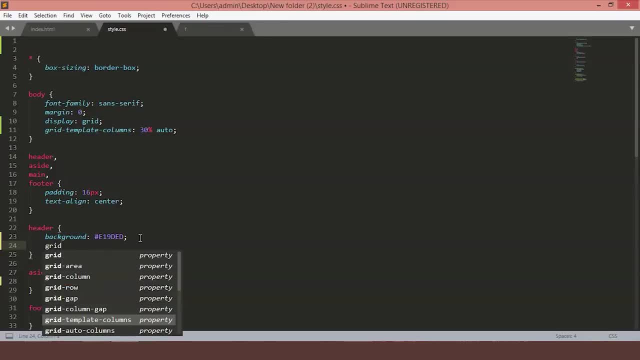 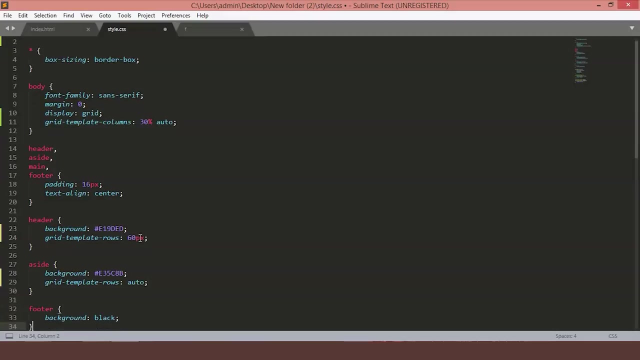 define the rows for our header and we will use the grid template rows. We will set the grid template rows for the header to 60px. For the sidebar and for the main content, we will set it to auto And also for the footer we will keep it 60px. 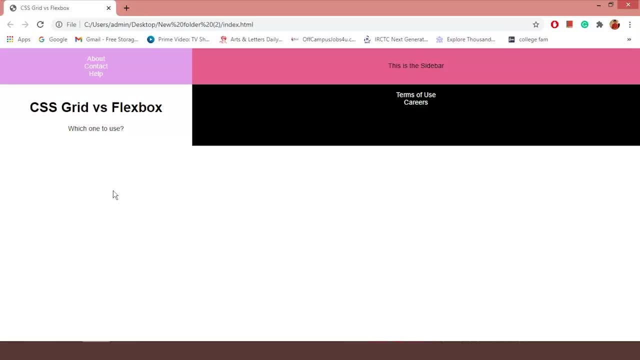 Now, if you save the file and reload, you can see the elements are adjusted in a 2D way, Just as we wanted. This shows the power of the grid and the flexibility it provides to the developer. However, we can see that the items are not positioned properly in the header and the 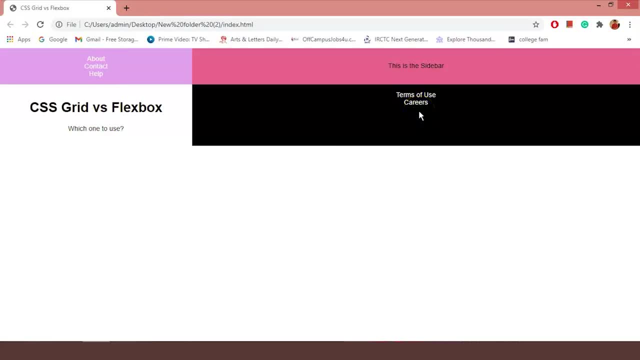 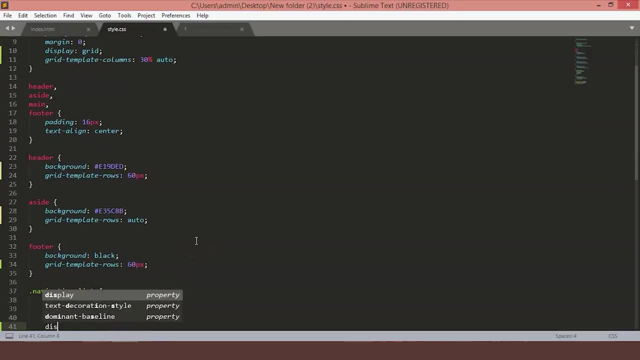 footer. This is where the flexbox comes into play. As discussed earlier, flexbox is about positioning elements in a one dimensional area, So what we will do is we will go back to our navigation list class here and we will add display as flex.